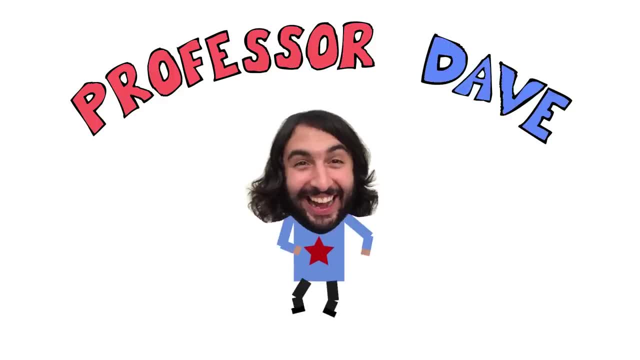 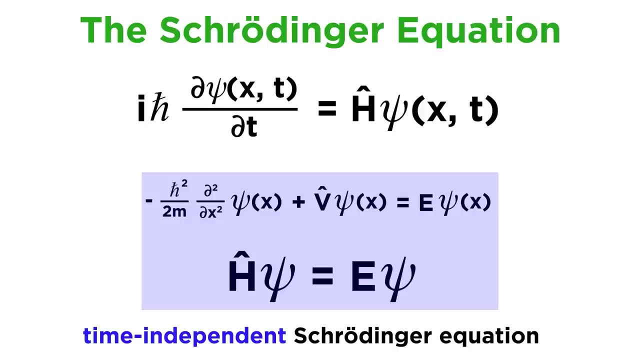 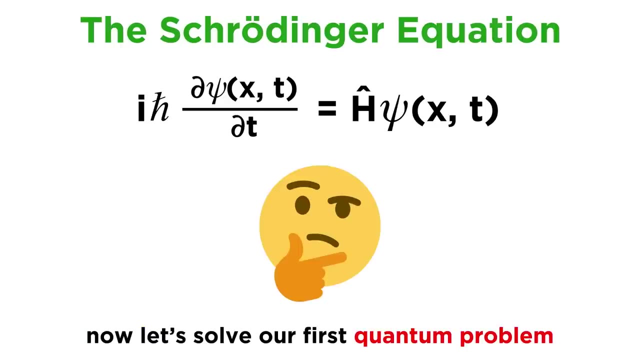 In the previous tutorial, we learned all about the Schrodinger equation. We derived different forms of this equation and talked about what all of them represent. Now it's time to apply this knowledge in order to solve our first quantum problem. This will be to find the 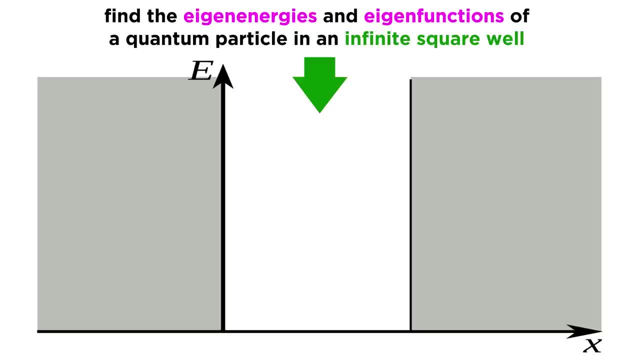 eigenenergies and eigenfunctions of a particle in an infinite square. well, This is also famously known as the problem of the particle in a box. We assume a potential which is as follows: V of x equals infinity everywhere, except between x equals zero and x equals a, within which 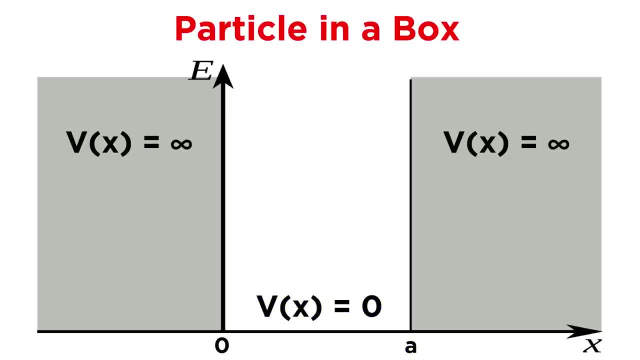 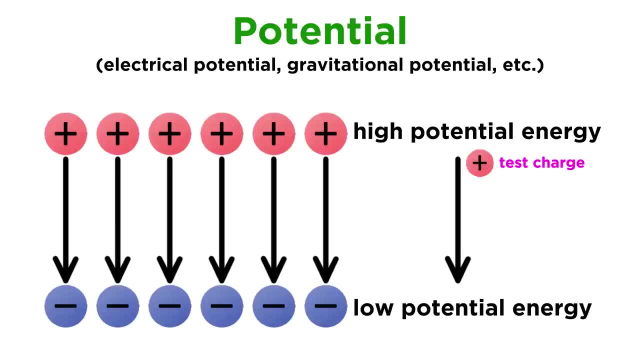 it equals zero. Let's unpack what that means a bit. We are probably familiar with the concept of a potential, like an electrical potential or gravitational potential, and we know that an object will have a tendency to go towards a lower potential. A ball will fall and a 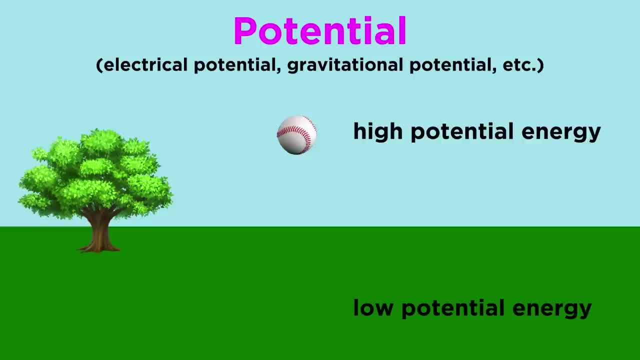 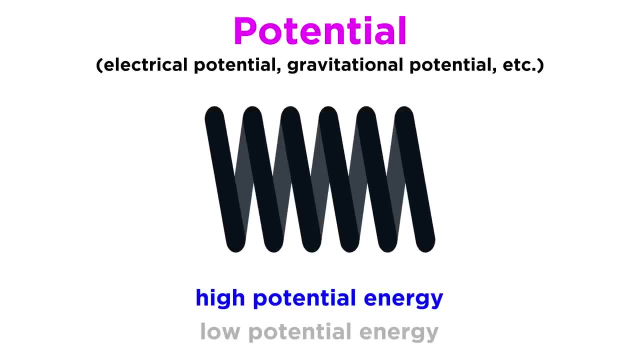 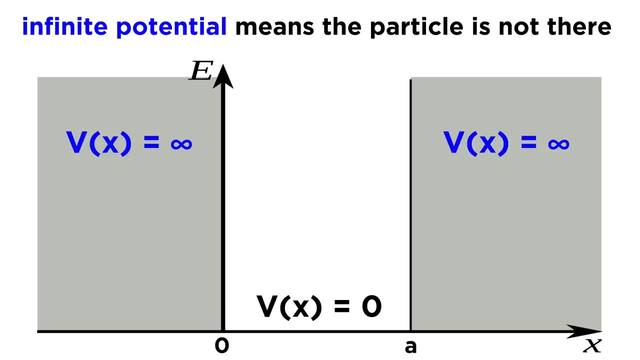 ball from some height, where it has greater gravitational potential, energy down towards the ground, its potential decreasing as it goes. A compressed spring will relax from a state of higher elastic potential to attain its equilibrium position. So here, when we say that V of x equals infinity for these intervals, this is the mathematical way of. 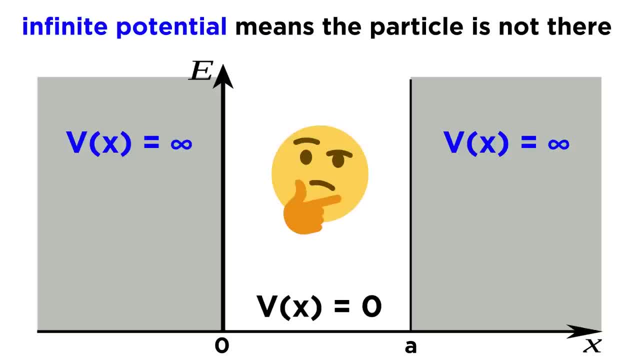 saying that the particle is definitely not there. That may seem counterintuitive, as it sounds like infinite potential should mean that it's certainly not there, But that's true. But remember that objects proceed towards a lower potential and infinity is the opposite. 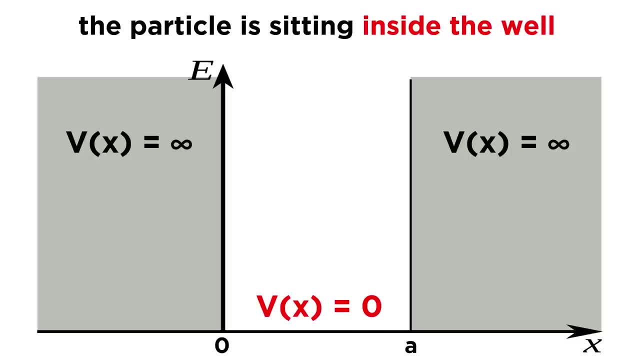 of that. So we know the particle is sitting in this square. well, The only thing is that, since we are looking specifically at a quantum particle, we have to use the Schrodinger equation to figure out where, or, more accurately, how, the particle lives within these walls. So 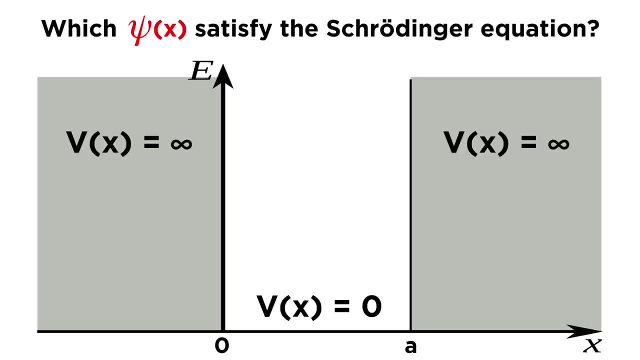 now what we want to do is to find the wave functions, psi of x representing this particle, which satisfy the Schrodinger equation. This is the same as asking what are the allowed states for a particle that lives between these walls? What does its probability, density function? 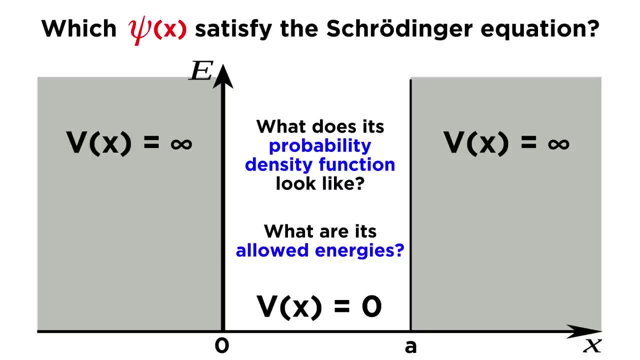 look like under these conditions, And also what are its allowed energies. All of these answers will arrive from determining which wave functions satisfy the boundary conditions imposed by the potential and the parameters imposed by the Schrodinger equation. The boundary conditions tell us something right away. The boundary conditions tell us that the potential 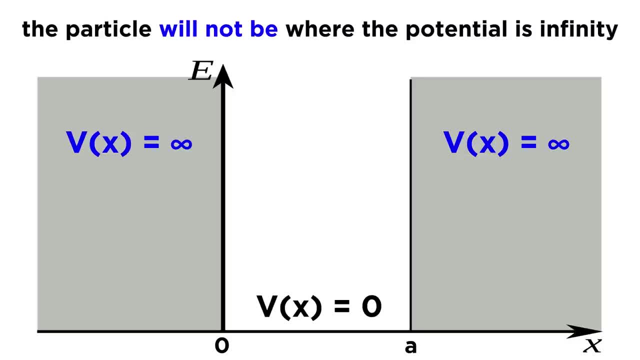 of the wave function is not the same as the boundary conditions imposed by the Schrodinger equation. As we said, the particle will surely not be located wherever the potential is infinity. That means that for those regions, the probability density function must equal zero. If the particle is not there, the probability of finding it there is zero, and the probability 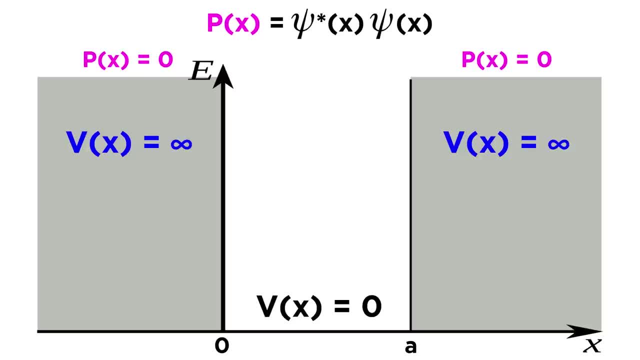 density function is equal to zero. The probability density function is psi, star times psi, so the only way for this to equal zero is for psi of x to equal zero. Therefore, we are looking for a wave function that will satisfy the boundary conditions imposed by the Schrodinger. 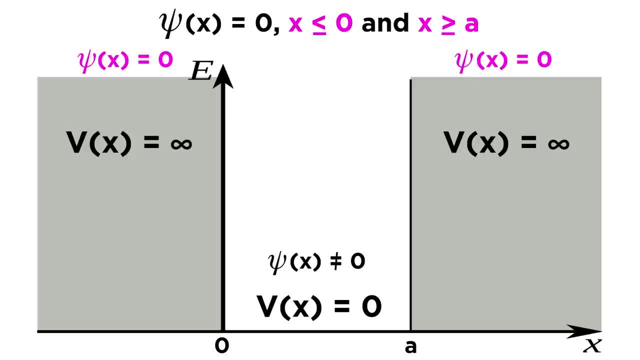 equation that will satisfy the following requirements: where psi of x equals zero, when x is less than or equal to zero, and also when x is greater than or equal to a, But between x equals zero and x equals a, the wave function does not equal zero and its 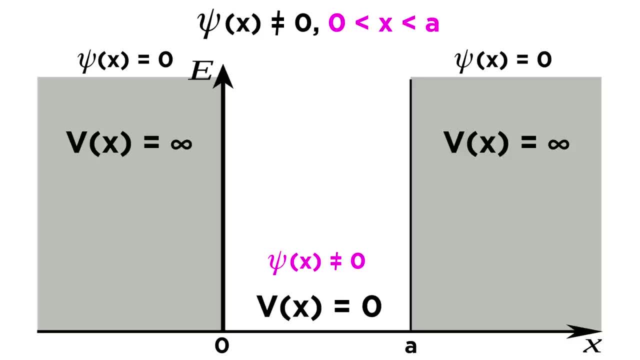 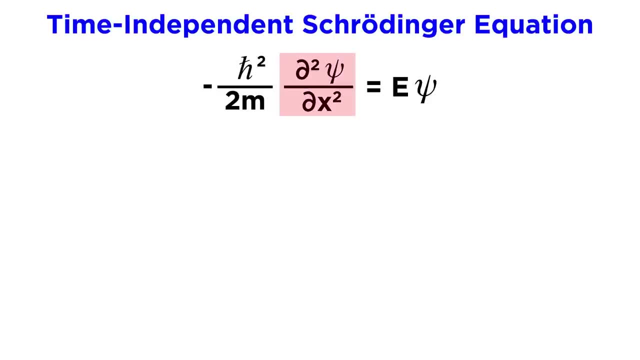 value can be determined using the Schrodinger equation. Let's use our new time-independent form of the equation, which, as we know, looks like this: We will find that isolating the partial derivative will make things easier. so let's move all of these constants to. 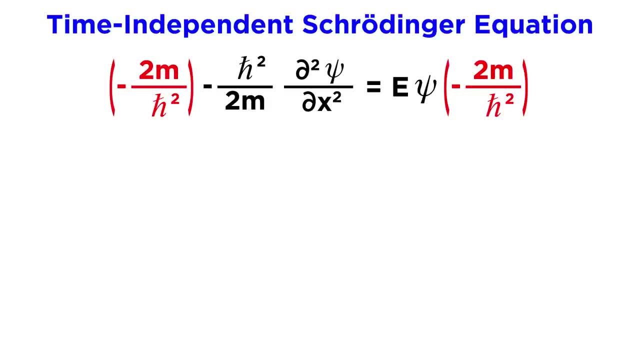 the other side, which will entail multiplying both sides by negative two m over h-bar squared. So now the second derivative of psi with respect to x is equal to negative two m e over h-bar squared times psi. Let's do another trick to simplify further. Let's define k as the 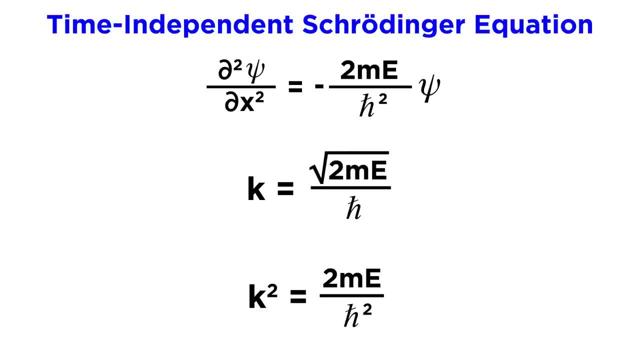 square root of two m e over h-bar, so that k squared is equal to negative two m e over h-bar squared. We can plug that into our equation to simplify the right side, which will now be negative: k squared psi. And finally, let's bring this term to the left side by: 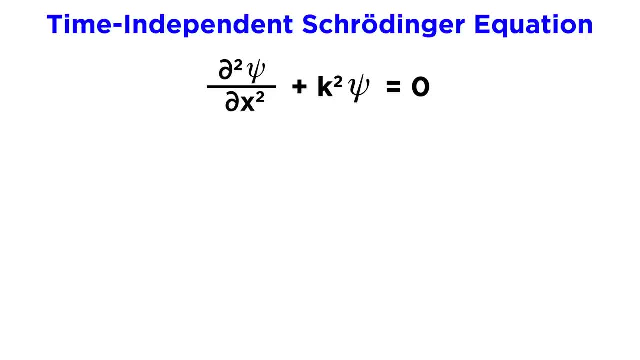 adding it to both sides. So we have the second derivative of psi. with respect to x plus k, squared psi equals zero. This is a second order differential equation which we need to solve in order to find psi. As we know, psi depends on x. Solving this differential equation entails finding all. 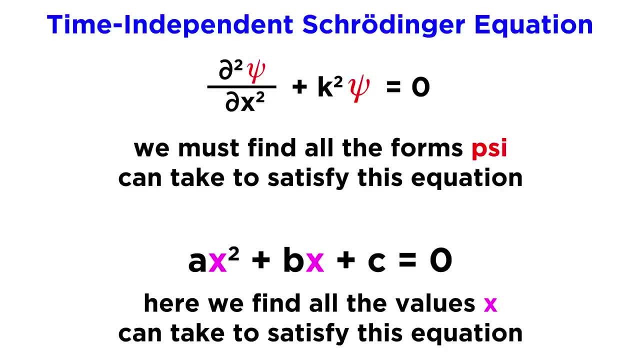 the forms that psi can take to satisfy this equation. just like solving a quadratic algebraic equation entails finding the values that x can take to satisfy the equation, There are simply different rules that must be used to find the solution. For example, if psi 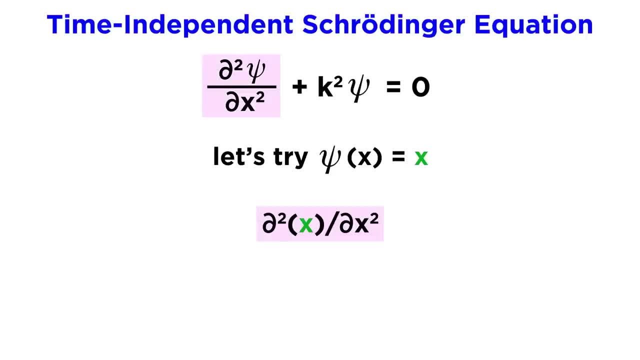 of x is equal to x, then when we take the second derivative of x with respect to x, the first derivative is one And the second derivative is zero. That leaves us with k squared. x equals zero, which can only be true if either k or x equals zero. K can't be zero because k depends on energy. 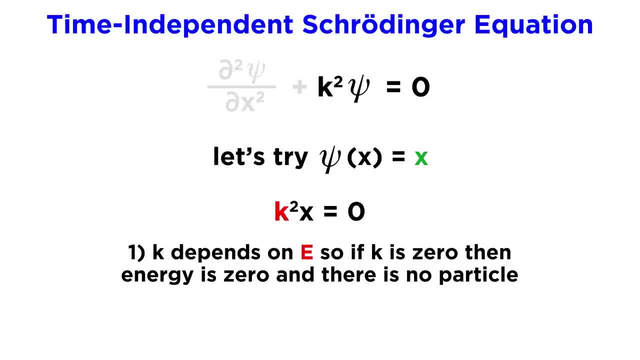 and if energy is zero, we don't even have a particle to begin with, And in this case, x can't be zero because psi equals x. Therefore, if x is zero, psi is zero and the probability density function equals zero, which we'll talk about in a bit. 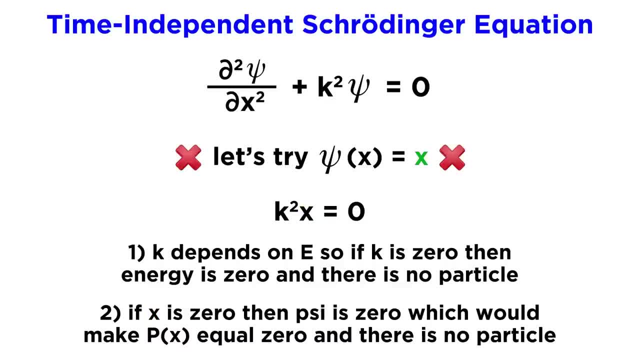 This whole thing once again means that the particle does not exist. So this is not a useful solution, because we know that there is a particle. this is a condition for the problem. So we would need to try something else Now. for brevity, rather than continuing to go through many possibilities, let's just: 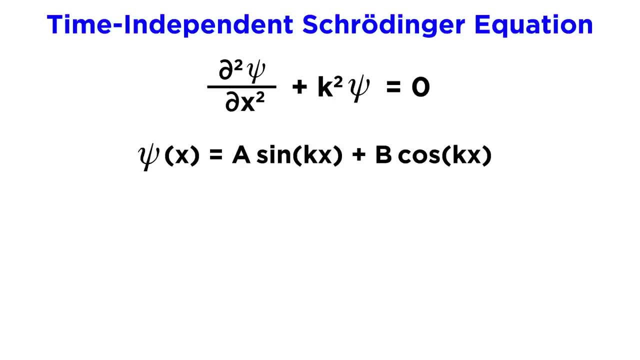 state outright that the solution to this differential equation is of the form: psi of x equals a sine kx plus b cosine kx. distance that we don't know yet but will determine by using the boundary conditions. And k is as we defined earlier. 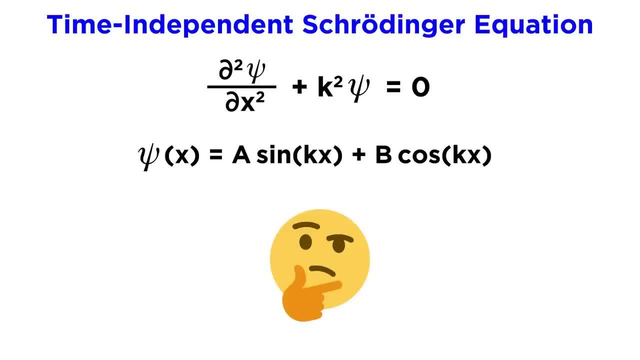 This may seem out of left field, but this general solution is arrived at through some clear-cut rules that are best omitted here to be covered over in the mathematics series for those who are interested. But this expression represents the solution of the time-independent Schrodinger equation. 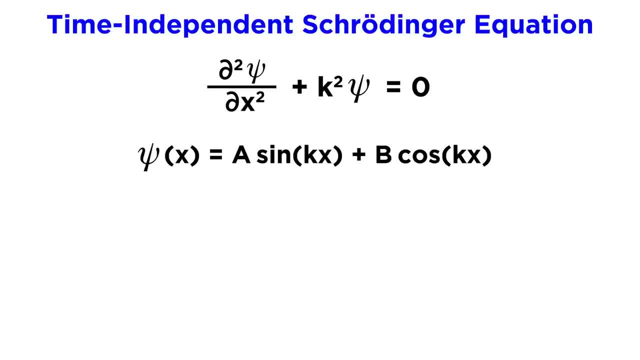 between the walls of the well. Just to quickly prove that this is the solution, we can plug this expression into our rearranged version of the Schrodinger equation. This first term involves taking the second derivative, So let's take the first derivative first. 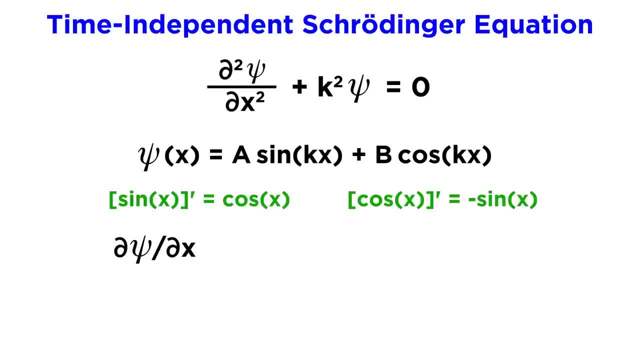 Remembering that the derivative of sine is cosine and the derivative of cosine is negative sine, and also that the chain rule requires that we bring k out front for each term. that will give us kA, cosine, kX minus kB, sine, kX. 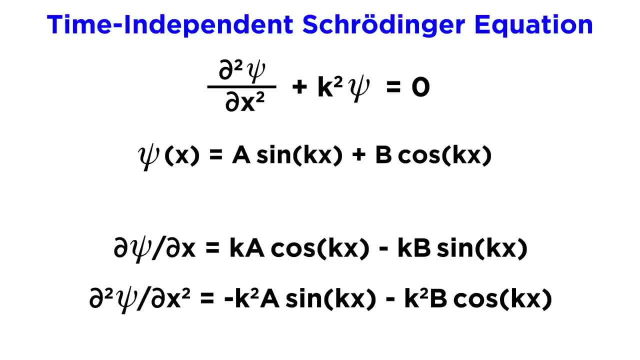 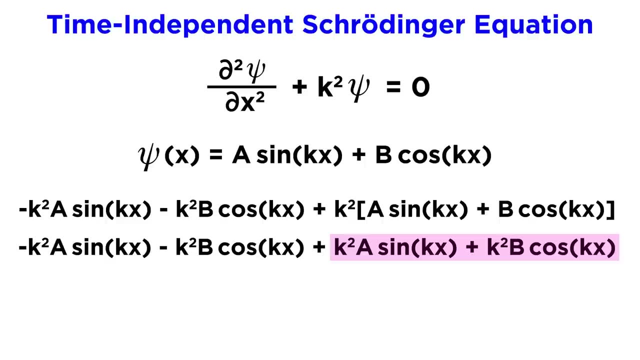 Okay, Then we take the derivative again and we get negative k squared A sine kX minus k squared B cosine kX. Then we add to that k squared times the original expression And distributing k squared we get k squared A sine kX plus k squared B cosine kX. 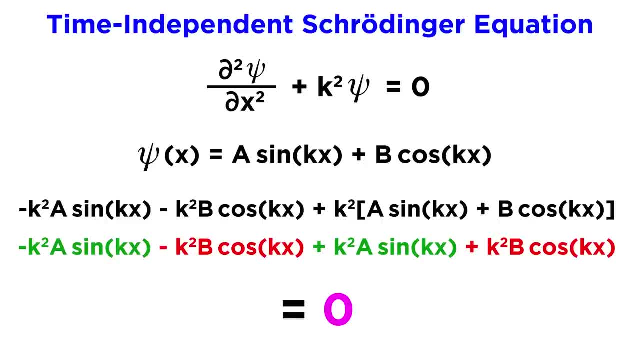 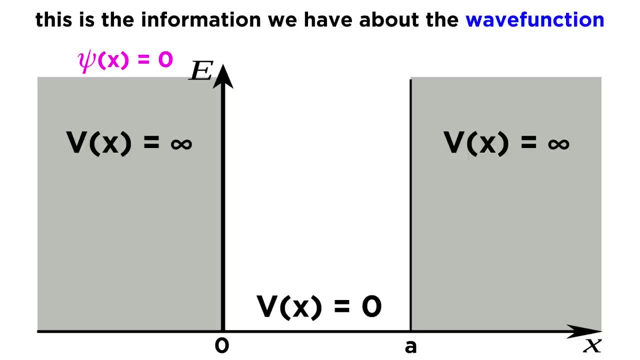 So, as we can see, everything cancels out to give us zero, as should be the case for any solution according to the Schrodinger equation. So, combining this with what we said before, psi equals zero. when X is less than or equal to zero, psi equals this expression when X is between zero and A, and psi again equals. 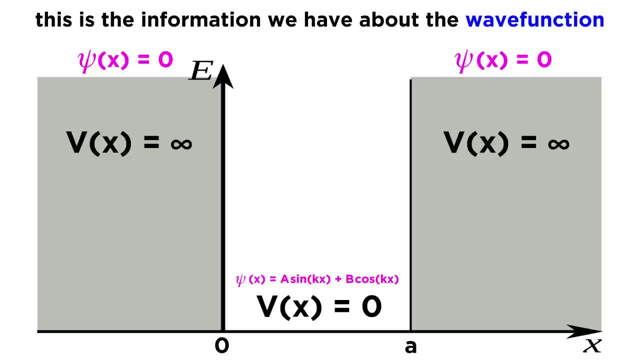 zero when X is greater than or equal to A. Let's now try to understand this graphically, as it will probably take us a while to figure this out. So let's take the derivative of sine k squared. A. sine kX minus k squared, B. sine kX plus k squared. 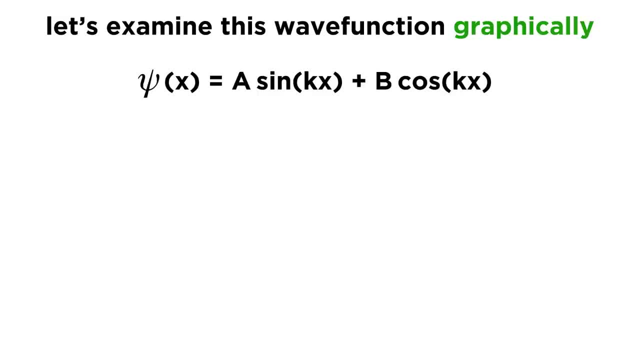 B sine kX plus k squared B sine kX. This will provide us with some understanding of the solution. As we said, the wavefunction must equal zero at the boundaries. This means that psi of zero equals zero And psi of A equals zero. 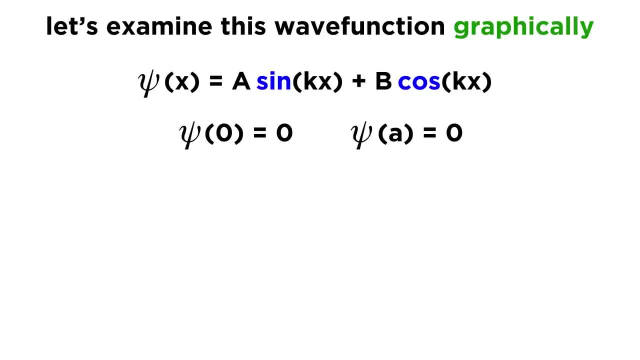 Now, since we have two different trigonometric functions to consider, it will be easier to examine them separately to get a sense of how they combine to give us the value for the wavefunction. Let's first remind ourselves of what sine of X and cosine of X look like. 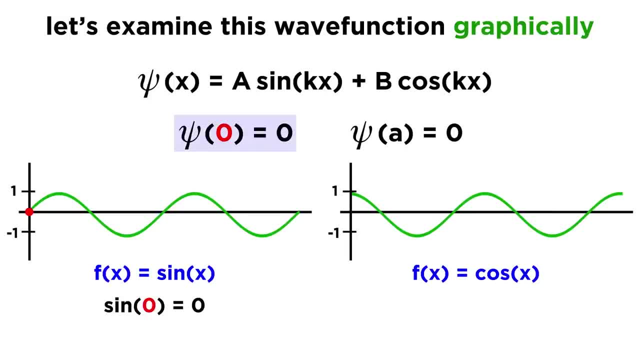 Let's first remind ourselves of what sine of X and cosine of X look like. What we need to notice is that sine of zero equals zero and cosine of zero equals one. This means that no matter what value for k we have in our expression, sine of k times. 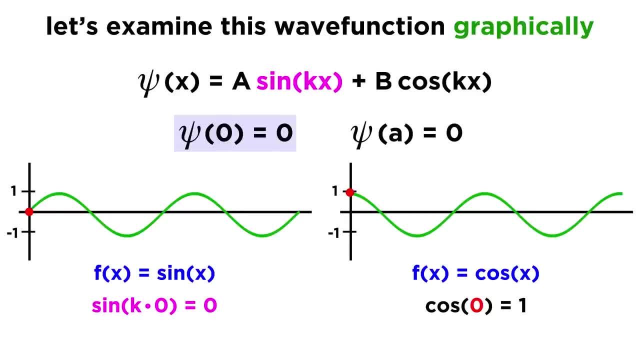 zero is still sine of zero, which will always be zero, and cosine of k times zero is still cosine of zero, which will always be one. This means that in order for their sum, in our expression, to equal zero, when X equals zero, The constant B must equal zero. 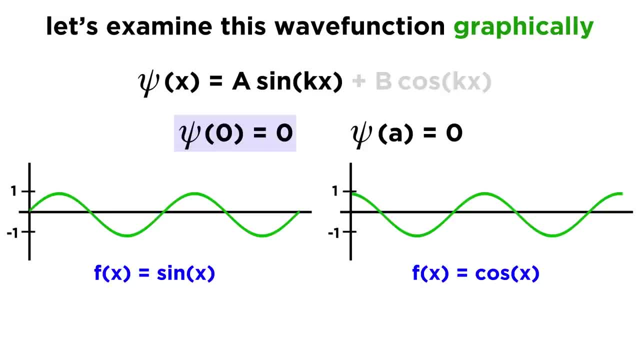 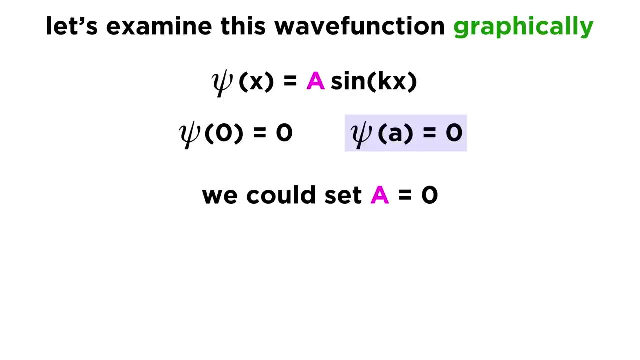 That means we can simplify our expression and get rid of the cosine term entirely. That leaves us with: psi of X equals A sine kX. Now let's examine the other boundary. Psi of A must also equal zero. This could be achieved by setting the constant A equal to zero, but that would mean that 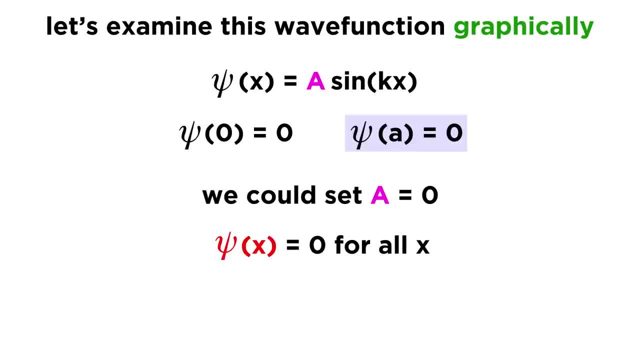 psi of X equals zero for all values of X. This again means that the probability density function would equal zero for all values of X and there is no particle. so that is not a useful solution. The other possibility is that sine of kX equals zero, and we are specifically examining the 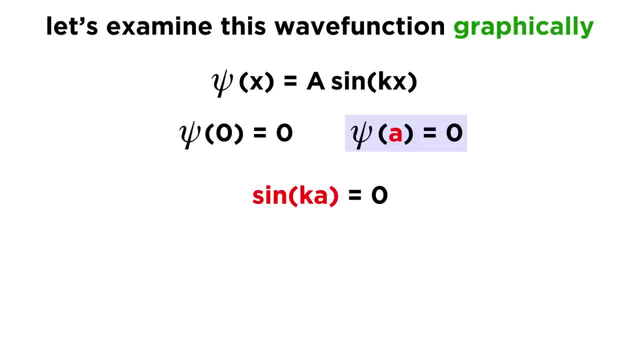 boundary where X equals A, so sine of kA must equal zero. Looking back at our graph of sine of X, we know that it is equal to zero. at X equals zero, and again at pi And two pi And every successive multiple of pi. 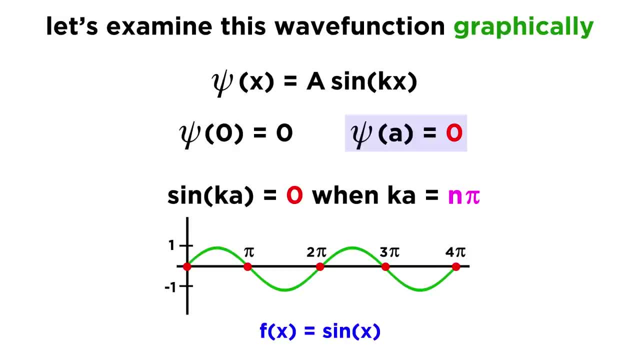 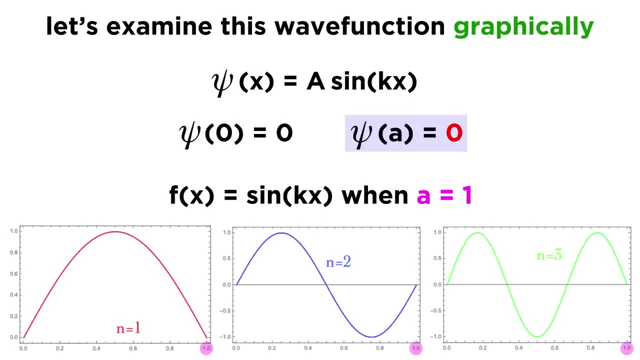 Therefore, sine of kA equals zero. when kA equals n pi where n is any integer, This also means that k equals n pi over A. Let's again examine this graphically. To make things simple, let's set A equal to one and then examine the graphs of sine. 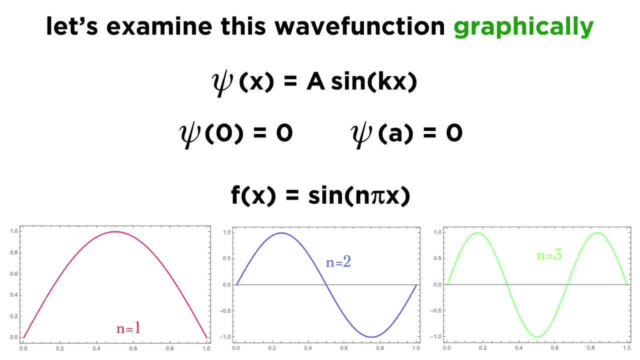 of kX, Which will therefore be sine of n? pi. And again, sine of kA equals zero. when kA equals n? pi, where n is any integer? Let's again examine this graphically. To make things simple, let's set A equal to one and then examine the graphs of sine. 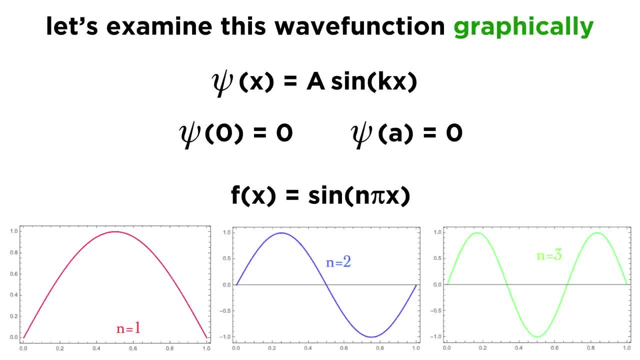 of kA equals n pi where n is any integer. And again, sine of kA equals n pi where n is any integer. And see what happens with different integer values for n. Each of these n values gives us a solution to the Schrodinger equation. 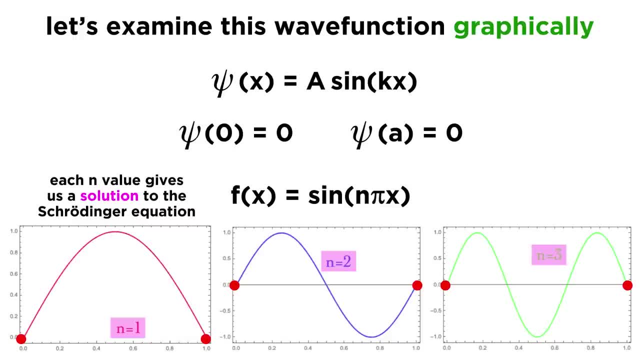 We can see that in each case, the wavefunction has a value of zero at both boundaries, Recalling that k depends on energy. if k also depends on n, then energy depends on n, and each value of n is giving us a different wavefunction or eigenfunction. 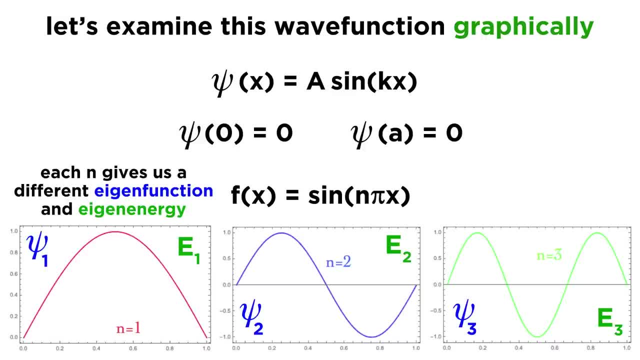 And a different eigenenergy for the particle. These are the allowed states for the particle. We can see how quantization comes into play here, as n must be an integer in order for the sine function, and therefore the wavefunction, to satisfy the boundary conditions. 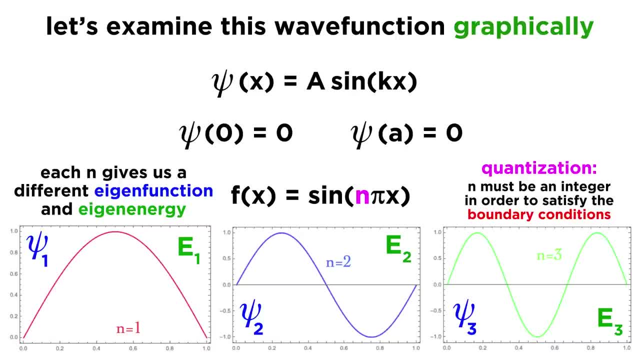 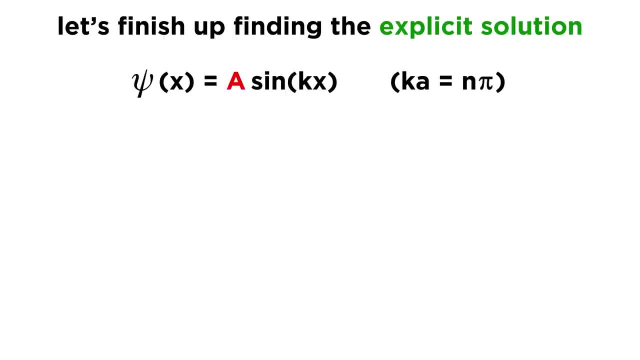 The fact that n must be an integer is what imposes quantization on this system. We have just one more thing to do: We have not solved for the constant a, so we still don't know precisely what the wavefunction looks like. In order to do this, the wavefunction must be normalized from zero to a. 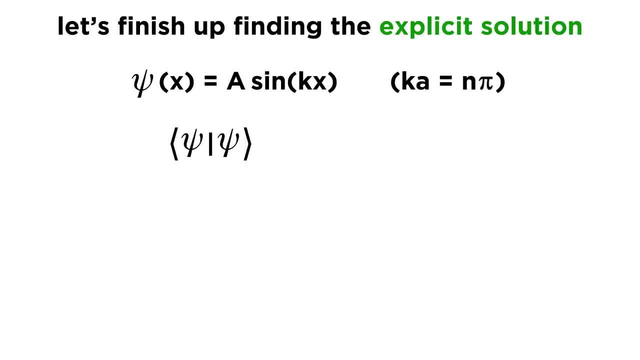 As we recall from a previous tutorial, we will use this braquette notation to represent the normalization of psi, which will equal the integral from zero to a of psi, star times, psi, dx, And because we are normalizing, this must equal one. Now, in this case, psi is a regular function. 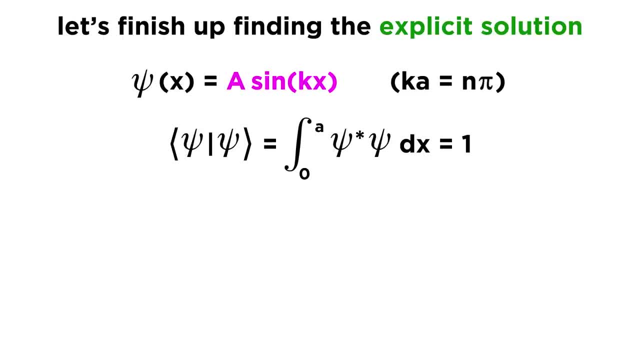 So we have to solve for the constant a. so we still don't know precisely what the wavefunction is. But psi is a real function. there are no imaginary terms. so psi, star times, psi is the same thing as psi squared. So let's just square our expression for psi and put that in the integral. 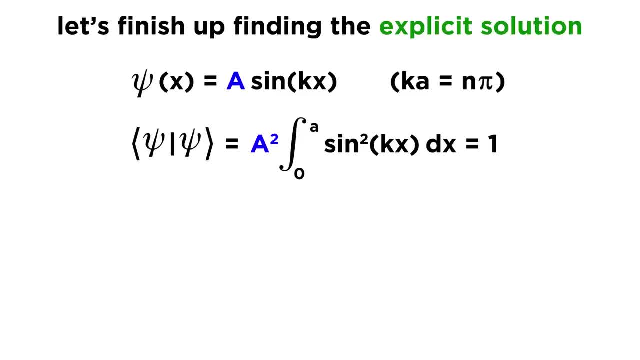 That gives us a squared, which is a constant, that we can pull out of the integral and inside the integral we have sine squared, kx, dx, which again must equal one. Now we have to solve this integral and if we are a little rusty with our integration, we will have to do this. 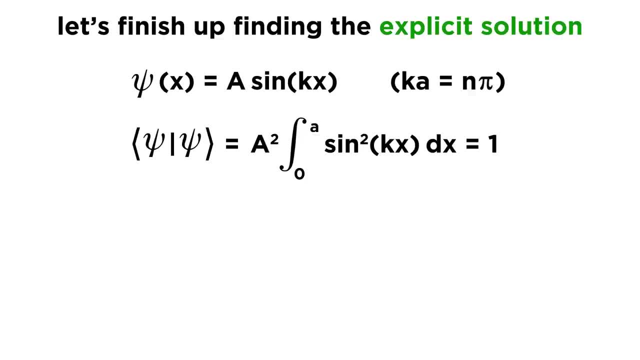 We have to remember that we can use a trigonometric identity here. Sine squared theta can be expressed as one minus cosine two theta over two. So let's apply that identity here and change our expression into one minus cosine two kx over two. 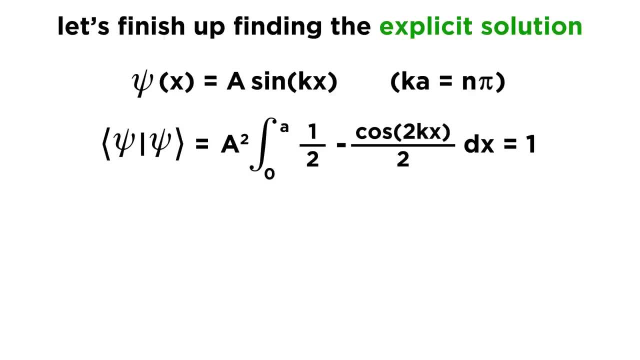 Let's make this simpler by splitting it into two terms and giving each its own integral. So the integral of one half dx minus the integral of one half cosine two kx over two, And we can evaluate these separately. The integral of one half is simply x over two. 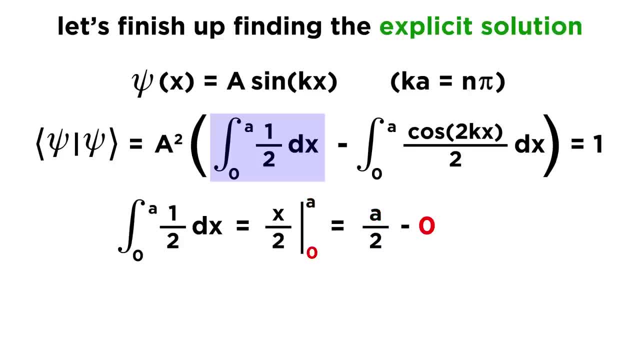 And plugging in our values, we get a over two minus zero or a over two. And the other integral isn't much harder, since we know that the antiderivative of cosine is sine. So we get sine two kx over two. 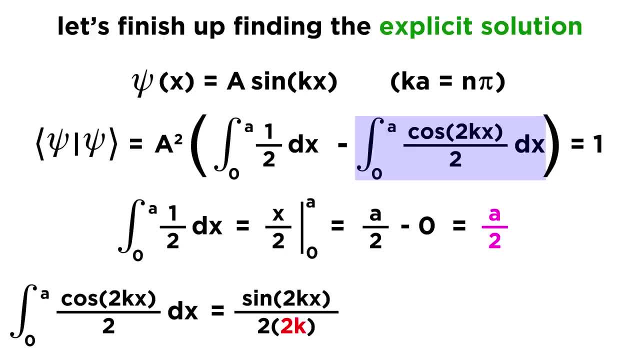 But then we have to put an additional two k in the denominator, because we are basically doing the chain rule in reverse And that will cancel out the additional two k in the numerator. that would occur if this were being differentiated. So now we plug in our values. 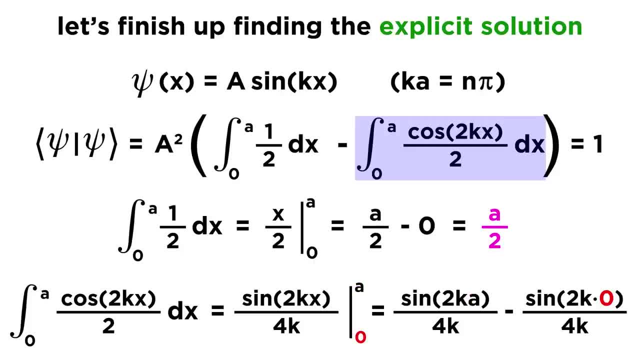 First we plug in a for x and then subtract from that the same expression, but with zero for x. Anything times, zero is zero and the sine of zero is zero, so this whole second term is simply zero. Now let's put the results of these two integrals in parentheses. 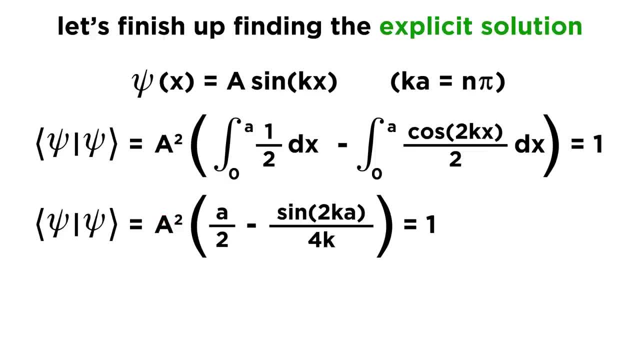 So that we can bring back a squared and then we can make another substitution. We know that k a equals n pi, so let's make that change. We know that n must be an integer, and we know that the sine of any multiple of pi must. 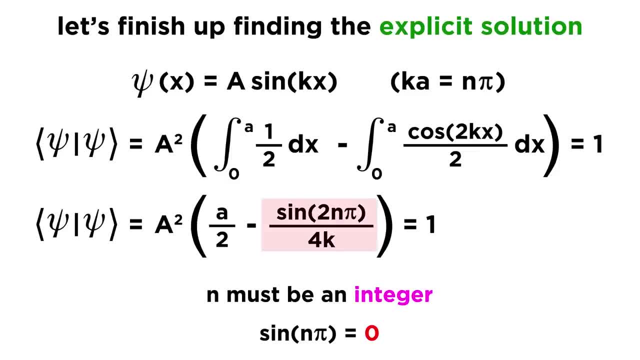 be zero, So this entire term will actually be equal to zero. That leaves us with simply uppercase A squared times lowercase a over two equals one, Just a bit more algebra. and we find that uppercase A must equal the square root of two over lowercase a. 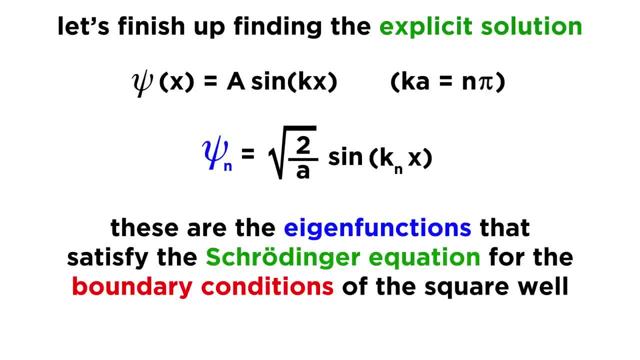 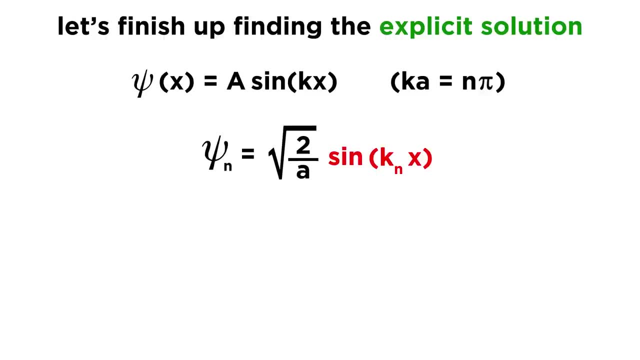 And now that we have solved for A, we can express our solution as a set of wavefunctions, which are the eigenfunctions that satisfy the Schrodinger equation for the boundary conditions given by the square. well, So psi sub n equals root two over a, sine k sub n times x. 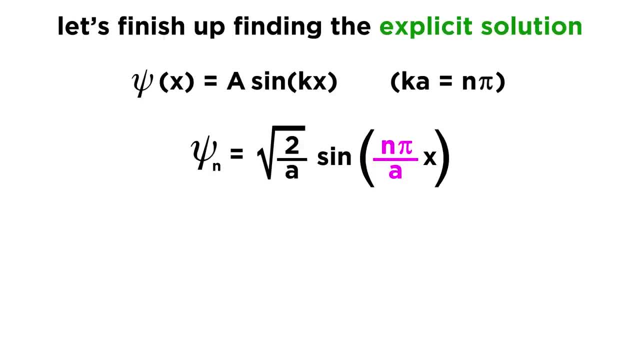 Where k sub n equals zero, Where k sub n equals n pi over a, where each integer value of n gives us a different wavefunction. So when n equals one, we get psi one. When n equals two, we get psi two. 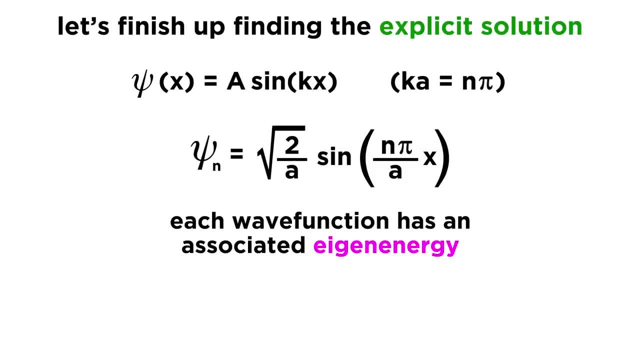 And so forth. Each of these wavefunctions has an associated eigenenergy. Using our definition of k, we can now express E sub n as being equal to h bar squared k sub n squared over two m. And given that k sub n equals zero, we can now express E sub n as being equal to h bar. 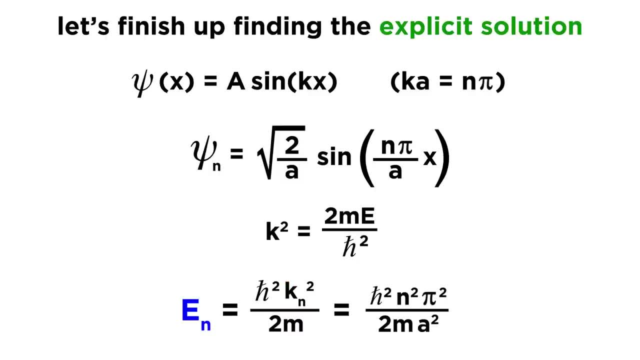 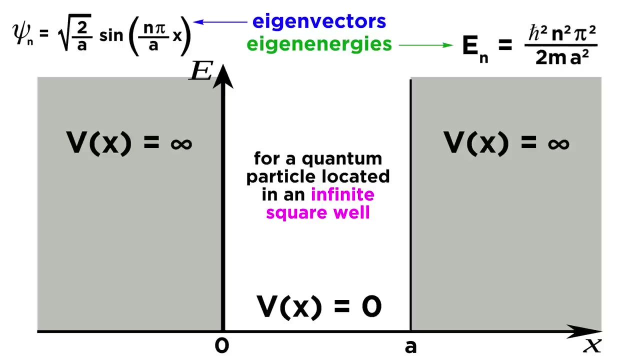 squared k sub n, squared over two m, Again, each integer value of n will give us an eigenenergy which describes the corresponding wavefunction. And there we have it. So that was definitely a bit of work, but we have successfully solved our first quantum. 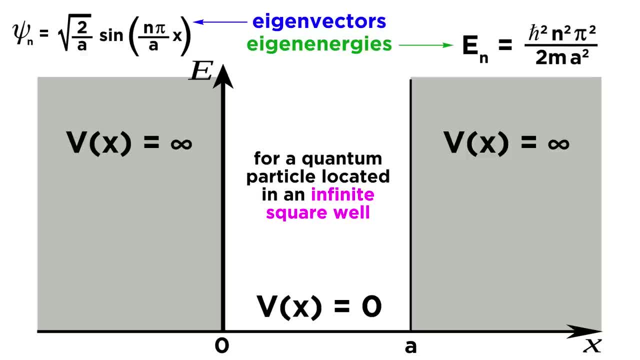 problem. We determined the allowed energies of a particle in an infinite square wavefunction. So that was definitely a bit of work, but we have successfully solved our first quantum problem. We determined the allowed energies of a particle in an infinite square wavefunction. 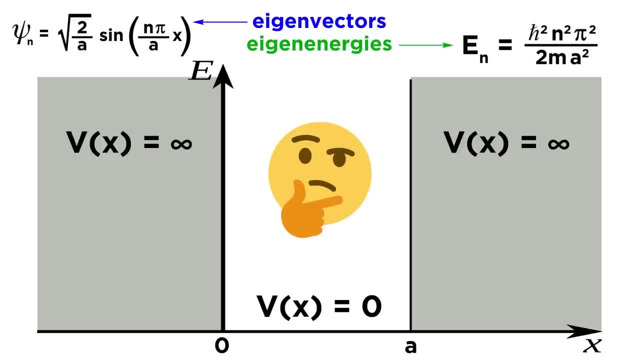 We determined the allowed energies of a particle in an infinite square wavefunction And, as if nothing else, we have been able to solve the problem in an infinite square. well, given certain boundary conditions. Even though the problem has been solved, there is still a lot to discuss in terms of the